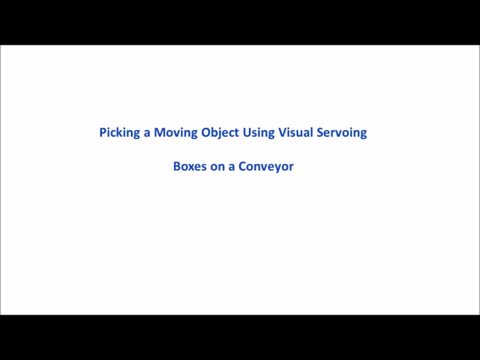 We'll be picking boxes from a conveyor belt that is not synchronized in any way with the robot. To pick a moving object, we have to identify it and instruct the robot to approach it with a known tool center position. We call this visual servoing. 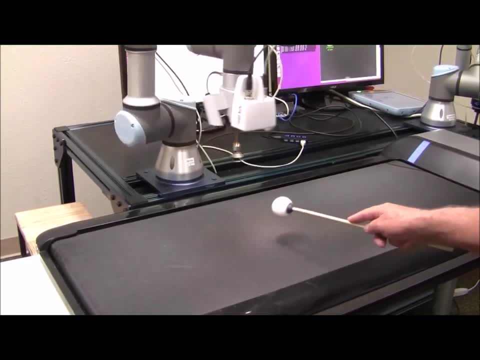 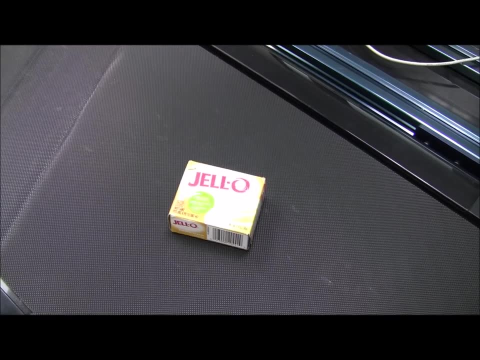 To illustrate the concept, here you see a robot following a moving golf ball in 3D space For our conveyor demonstration. the object we'll pick is nothing special: It's a jello bar. What's different is that we'll randomly orient these and place them on a conveyor moving at 250 mm per second. 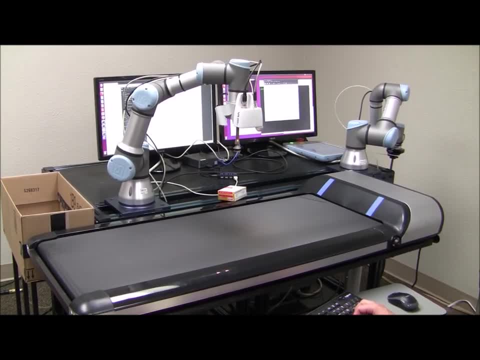 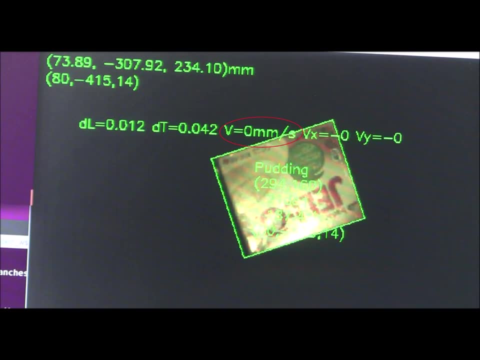 The robot will then visually locate them, pick them up and place them in the box. you see at the left. We've set the box on the conveyor. with the conveyor turned off, Our object finder locates it and identifies the velocity at which it is moving: 0 mm per second. 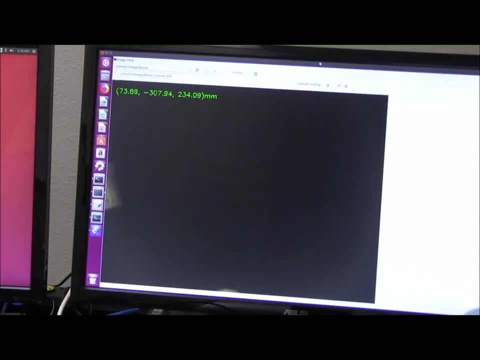 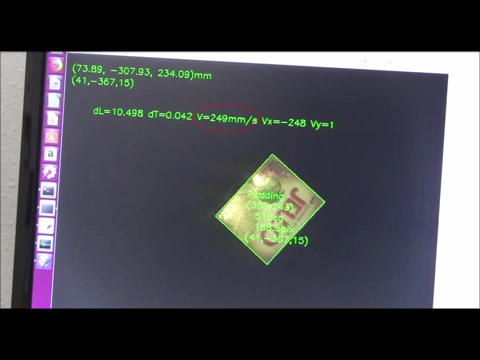 Now let's turn the conveyor on. As each box passes the camera, you can see its velocity on the screen. If we freeze the frame, you can read the velocity clearly. So we've located our object and detected its velocity without any conveyor instrumentation. 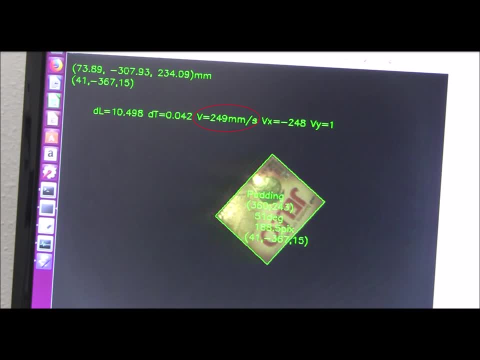 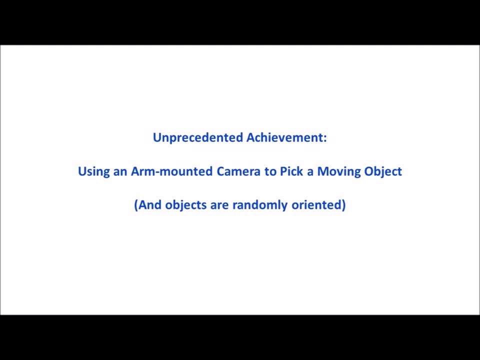 Our vision system is detecting the motion on its own and it has the information it needs to direct the robot to pick up the box. We've never seen an arm-mounted camera guide a robot to pick up a moving object. We believe this is an industry first. 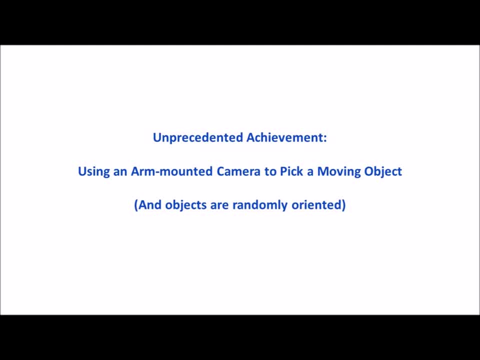 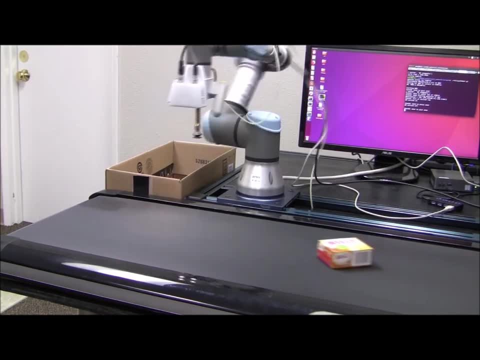 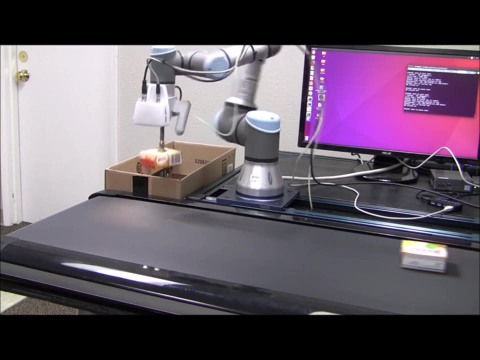 The camera and the objects to be picked are both in motion. Let's watch. Notice that the boxes are oriented every which way, at varying intervals and various placements on the conveyor, And yet the vision system consistently locates them and completes the pick. Also, notice how fast this operation runs. 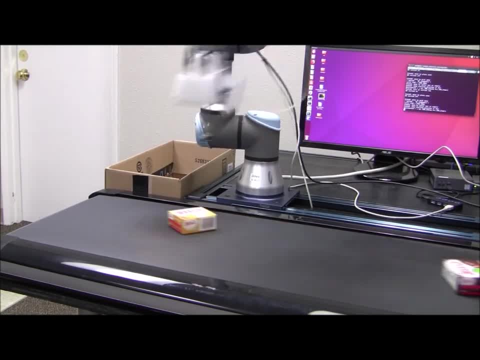 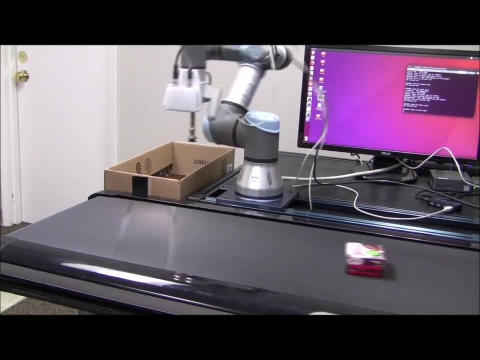 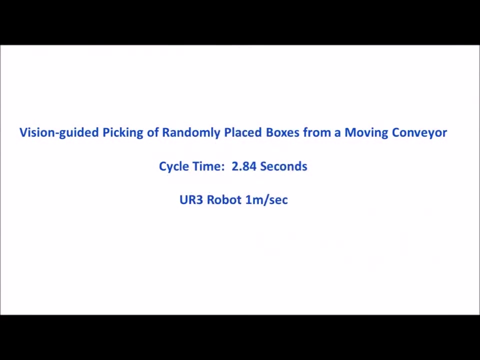 This is a 1 m per second UR3 robot, not some 4 m per second industrial robot, And yet our average cycle time is under 3 seconds. To be more precise, our average cycle time is 2.84 seconds and we are working on additional path planning optimization that will cut that time down even further.